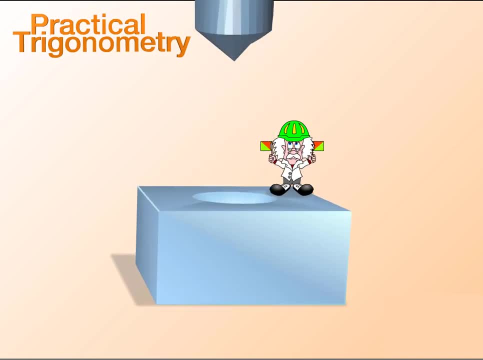 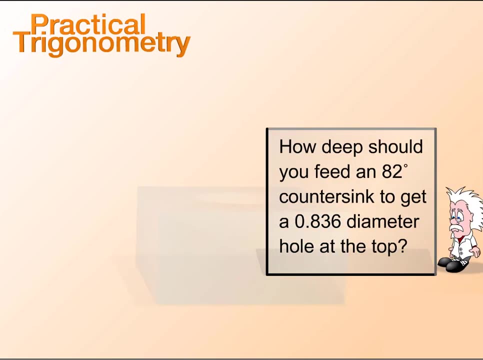 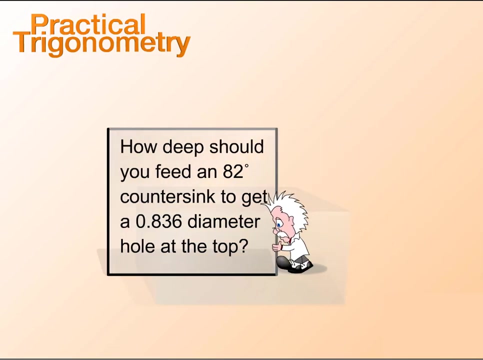 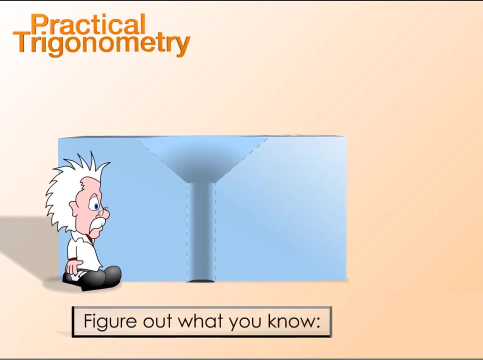 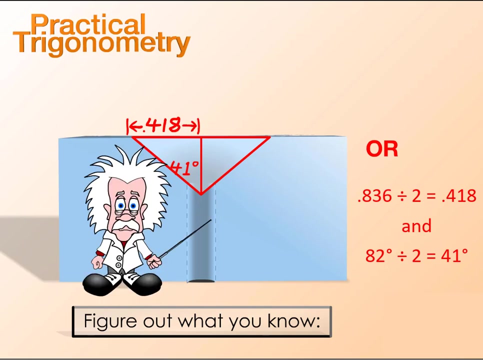 How deep should you feed an 82-degree countersink to get a 0.836-inch diameter hole at the top? Figure out what you know, Draw and mark a diagram as shown. Once you know your measurements, label the sides of the triangle according to the angle. 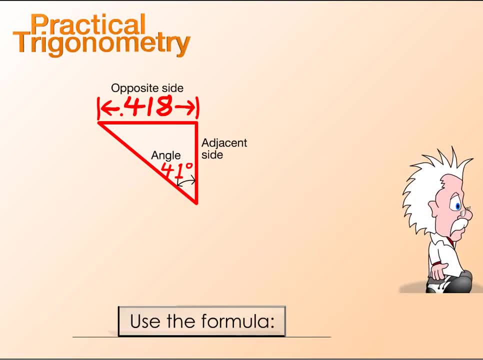 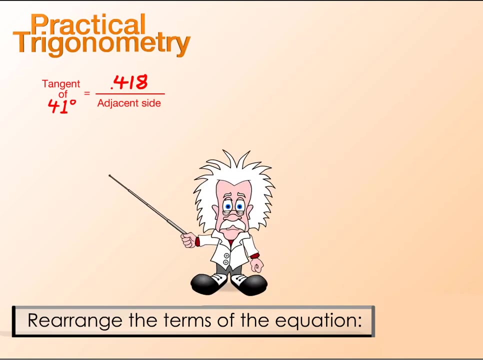 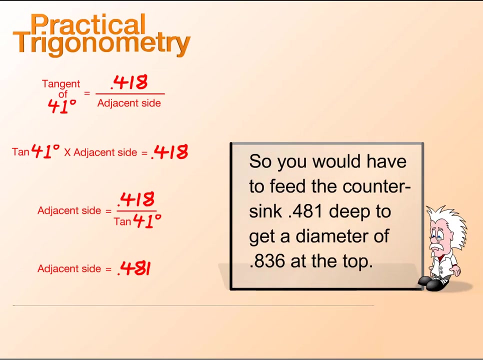 you are using In this example. use the formula: tangent of the angle equals the opposite side length divided by the adjacent side length. Use algebra to rearrange the terms of the equation and solve as shown. So you would have to feed the countersink 0.481 inches deep to get a diameter of 0.836. 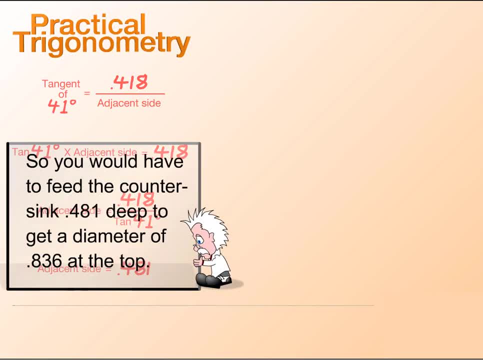 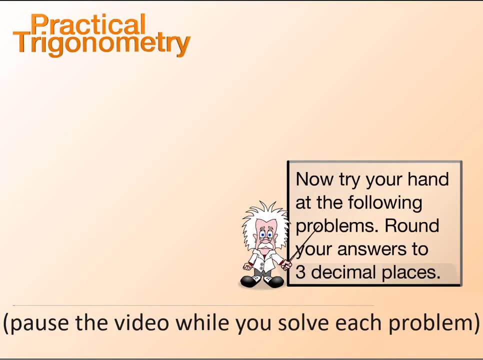 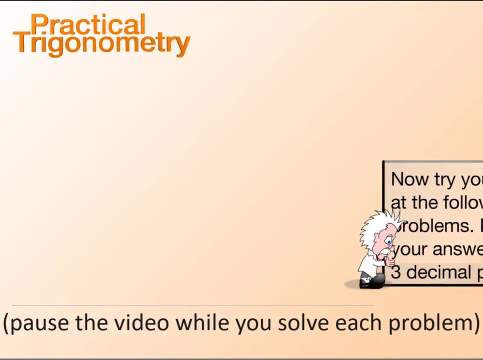 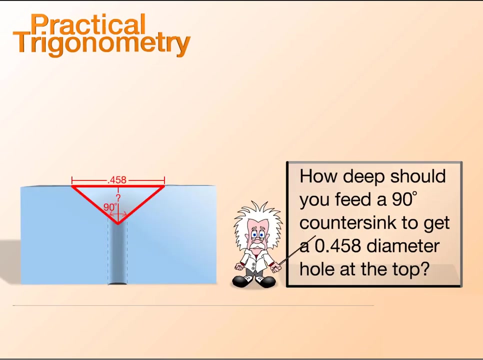 inches at the top. Now try your hand at the following problems. Round your answers to three decimal places. Pause the video while you solve each problem. How deep should you feed a 90-degree countersink to get a 0.458-inch diameter hole at the top? 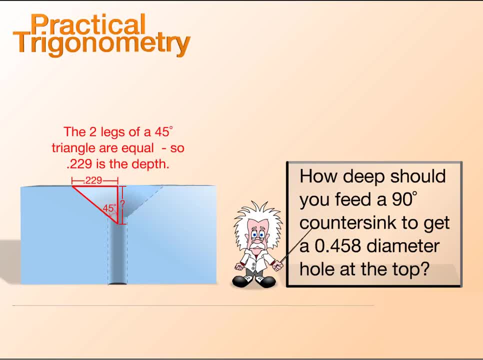 Now watch as the problem is solved. The two legs of a 45-degree triangle are equal, so 0.229 inches is the depth. If you use tangent, as in the example, you should get the same result. This is a shortcut for 45-degree right triangles. 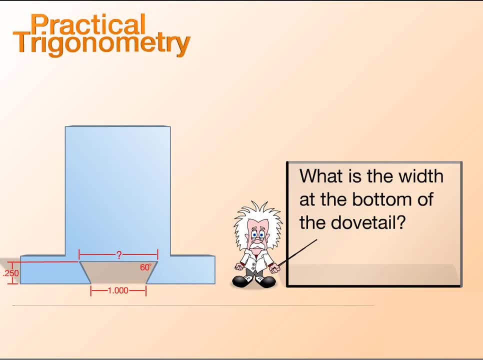 What is the width at the bottom of the dovetail? Watch as we solve for the adjacent side. Remember to add it to both sides of the 1-inch length, as shown. So the total length of both sides of the 1-inch length is shown. 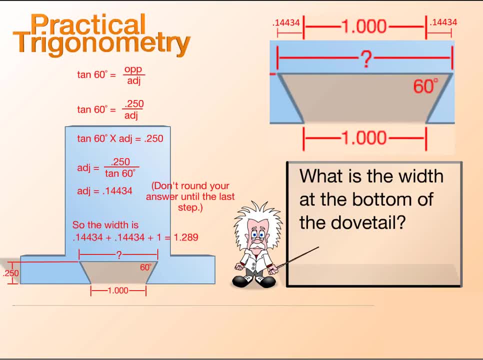 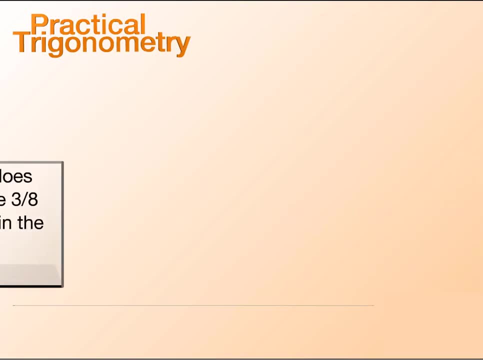 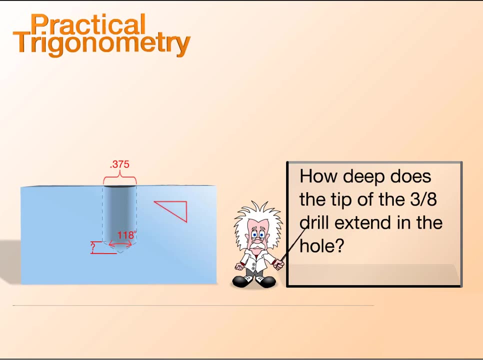 So the total length of both sides of the 1-inch length is shown. The total width is 1.289 inches. How deep does the tip of a 3-eighths-inch drill extend in the hole? Watch the solution for the adjacent side. 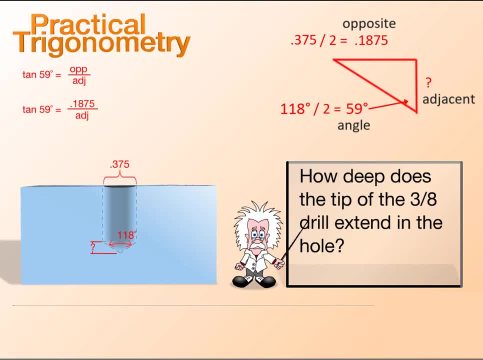 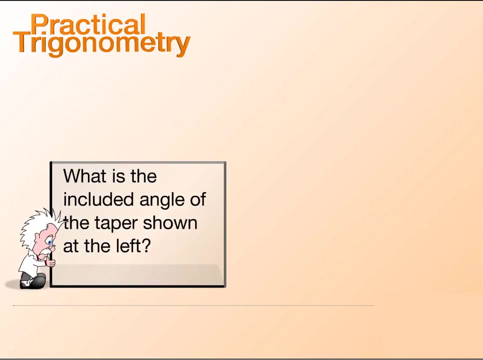 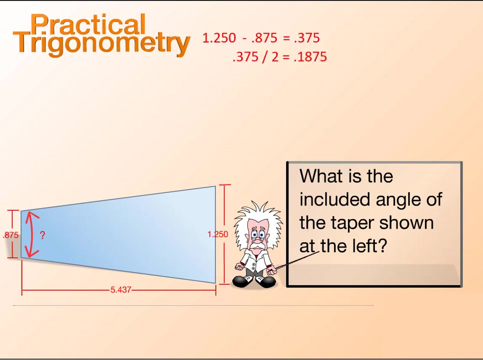 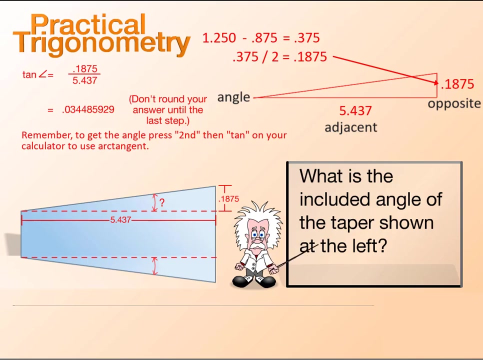 So the tip of the drill extends 0.113 inches into the hole. What is the included angle of the taper shown at the left? Watch as we solve for the angle. Remember to get the angle. press 2nd, then tan on your calculator to use arctangent. 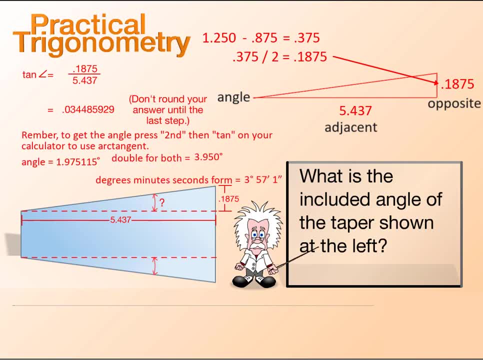 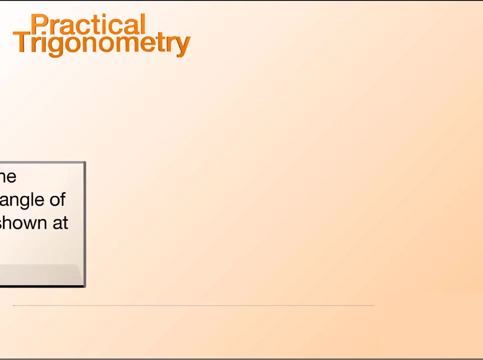 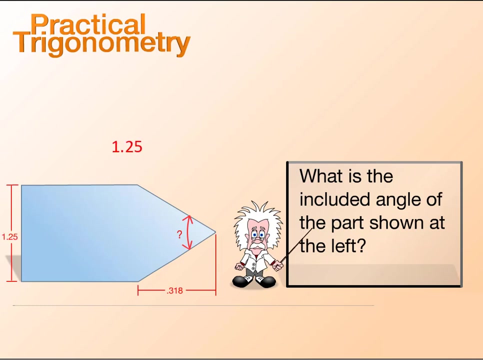 We need to add both angles together, so double the answer to get 3.950 degrees or 3 degrees. 57 minutes, 1 second. What is the included angle of the part shown at the left? Watch as we solve for the missing angle. 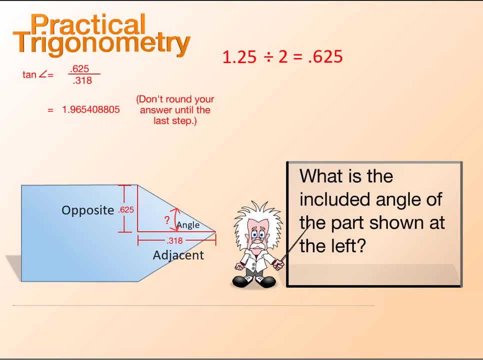 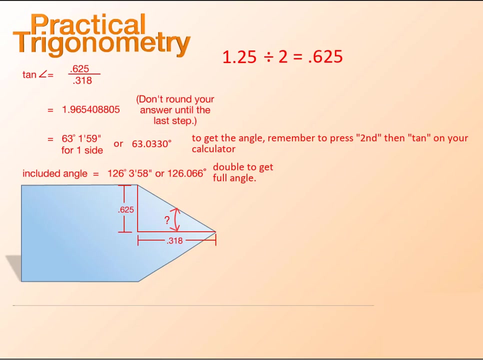 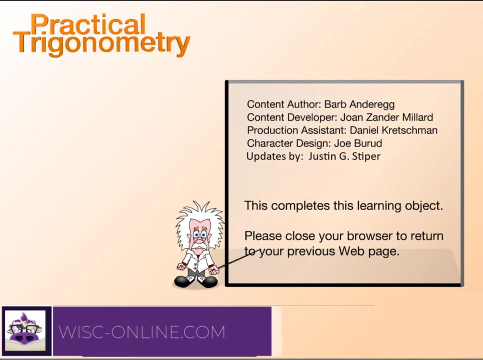 The full angle is 126 degrees. 3 minutes 58 seconds or 126.066 degrees. This completes this video. Practical Trigonometry. Thank you for watching. 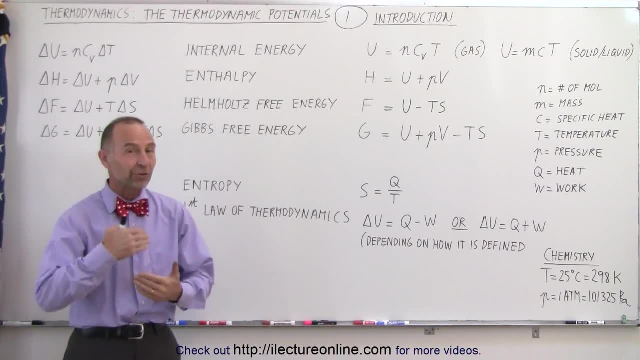 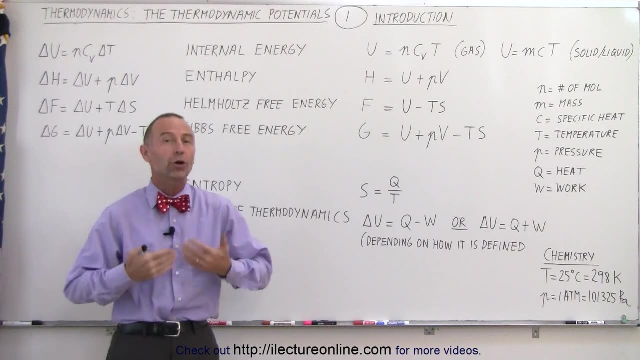 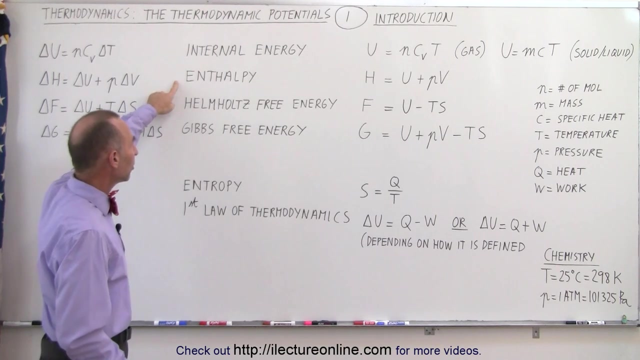 Welcome to our lecture online. In this video and the videos to come after this, we're going to talk about the thermodynamic potentials, And the question, of course, is: what are the thermodynamic potentials? Well, there are four of them, and they are as follows: The internal energy, the enthalpy. 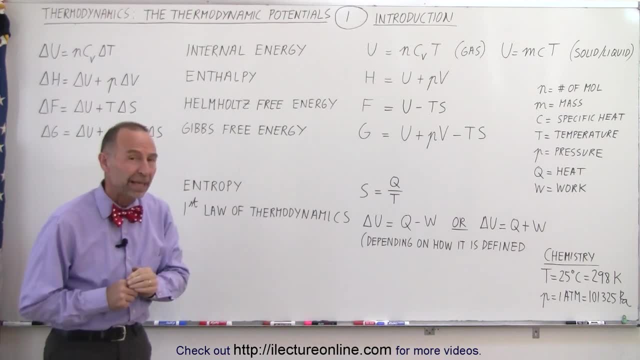 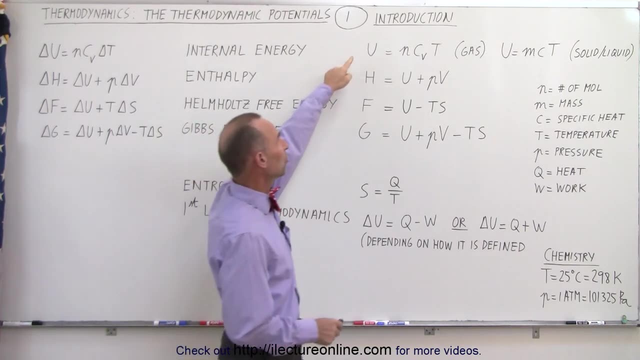 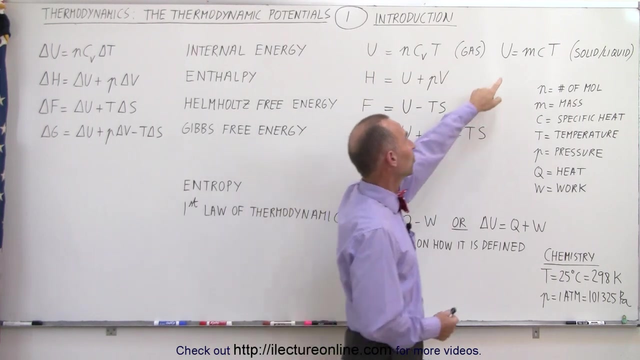 the Helmholtz free energy and the Gibbs free energy. And here, if you look them up, are the equations that will define the four thermodynamic potentials. Notice that the internal energy can be defined in terms of, if it's a gas- N, C, sub V, times, T- And in terms of a solid or liquid. 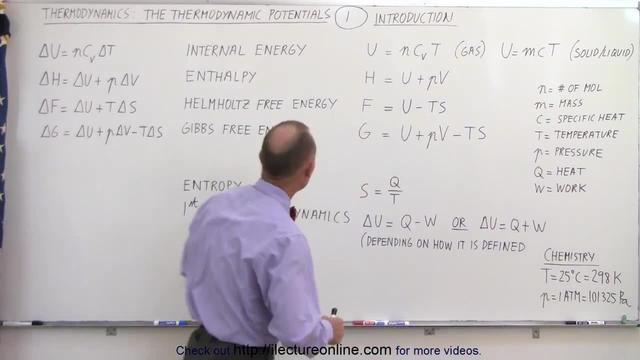 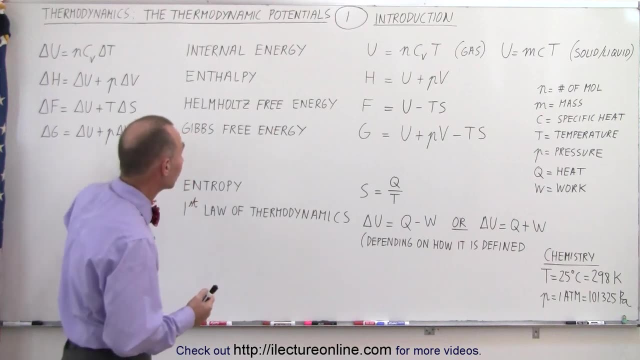 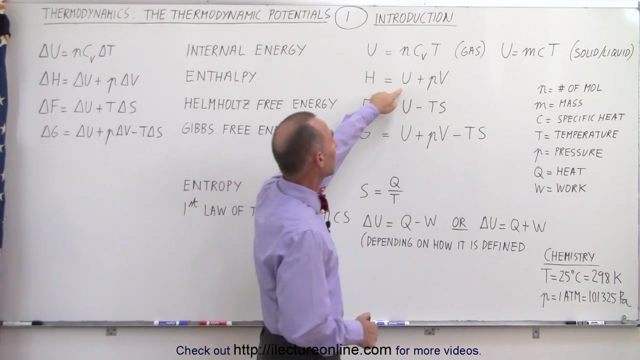 U equals MC times T. Notice there's a set of equations on the left side here where we have it in terms of the change in, And those are much more practical most of the time than these equations right here, although we need both sets. The enthalpy is defined as the internal energy. 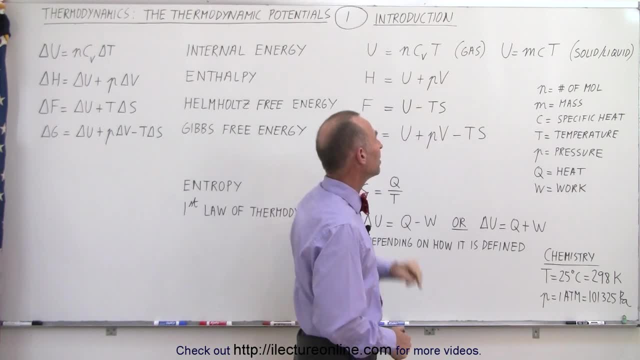 plus P times V, P being the pressure, V being the pressure, And the energy is defined as the volume. F, which stands for the Helmholtz free energy, is equal to the internal energy minus T times S. S is the enthalpy and T is temperature. And finally, the Gibbs. free energy is defined as 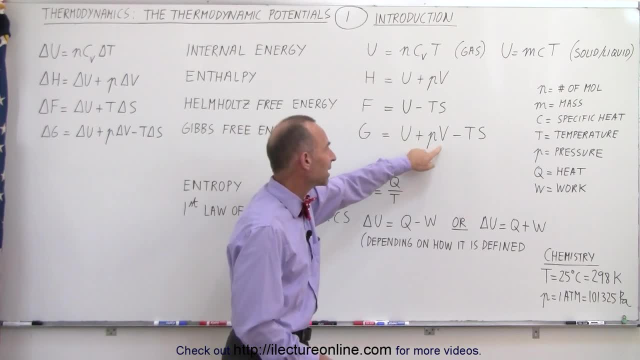 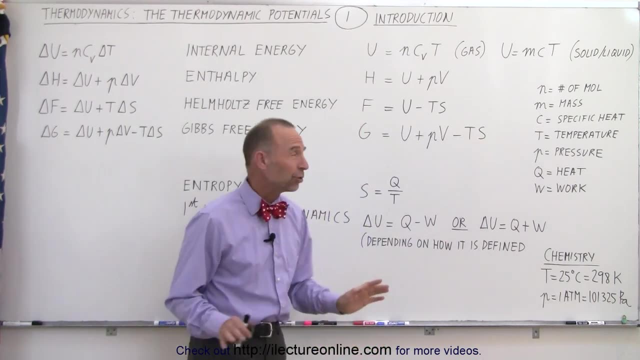 the sum of U- the internal energy- plus P times V- the pressure times, the volume- minus T times S, which is the temperature times, enthalpy, And I know you see this and go. I've seen these equations before and I have no idea what they mean. And that is the typical.